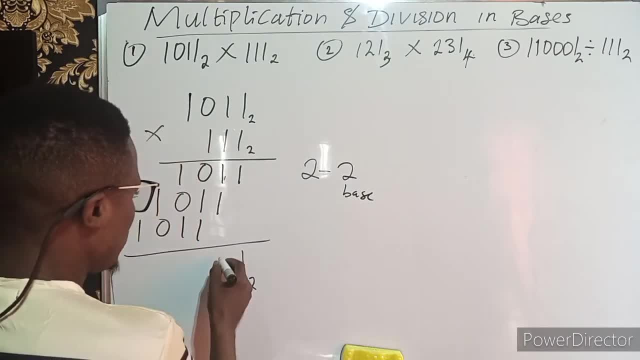 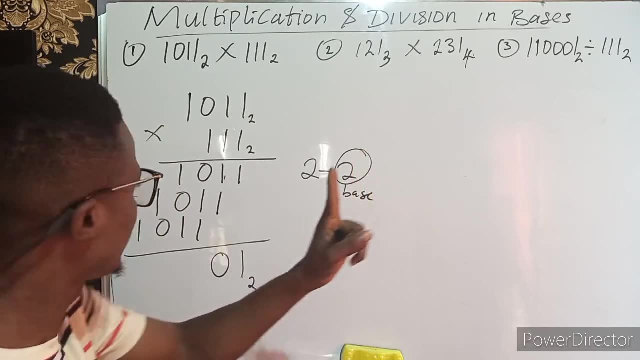 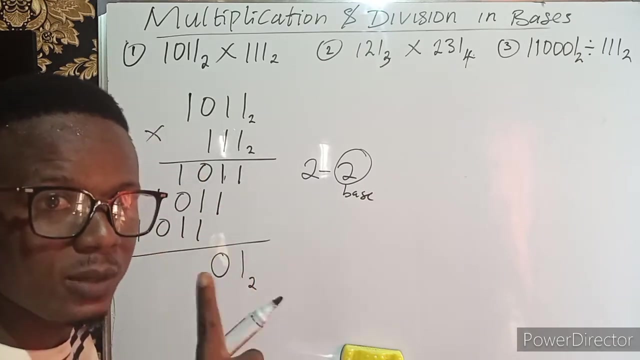 base two. this one is the base that will give me zero. but this base two i have minus. i'm not going to throw it away. i'll call it one whole bundle. that one bundle i'll carry it over here, so i'll that. base two means two, which is one, one. two in base two is one, so i'll carry that, uh, one. 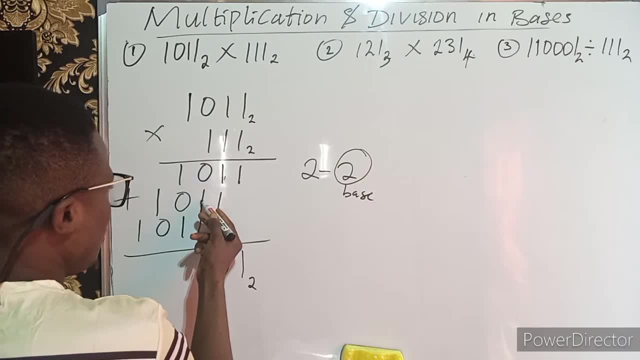 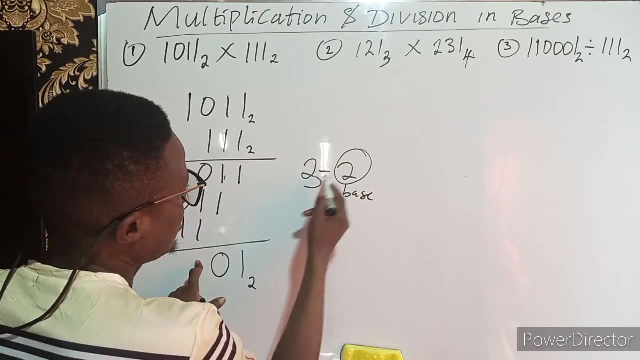 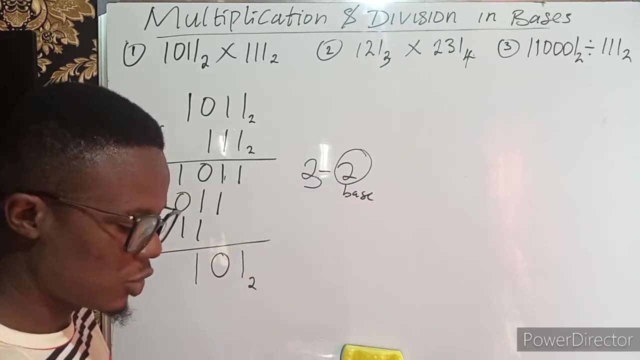 and place it here. one plus zero is one plus one. two plus this one, three again. i'm not allowed to write three, that three. i will say three minus the base two again. that will give me one. the base two are minus. i will call it one. i shouldn't throw it away again. i will transfer it over here again. 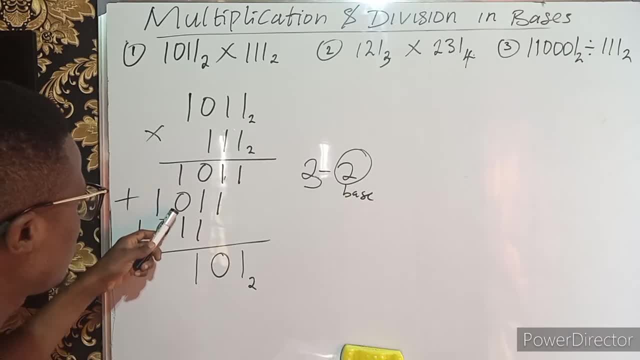 that one plus this one is two, two plus zero is two and two plus one will give us three. i'm not allowed to write three again. you three minus base two is still one. the base two i have minus, i'll carry it over that is as one. that one plus this one is two and two plus zero is two. i cannot write two. i will. 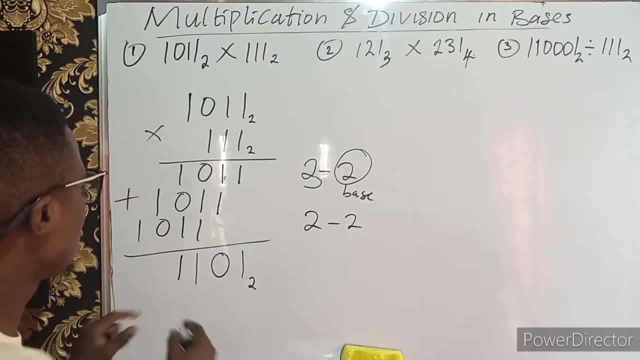 still say two minus the base two. of course it will give me zero. the base two i have minus. i'll call it one again. transfer the one to this one, it becomes a two. i cannot write two. also, i will still say two minus base two, which is a zero. 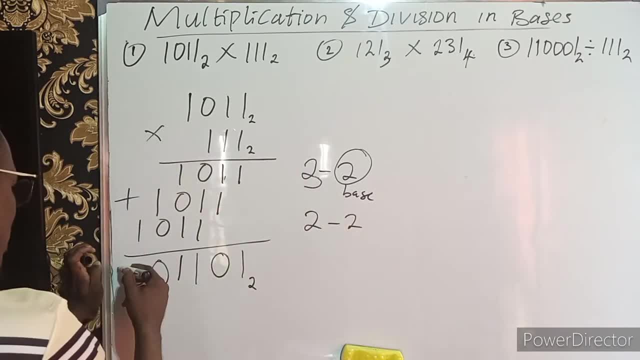 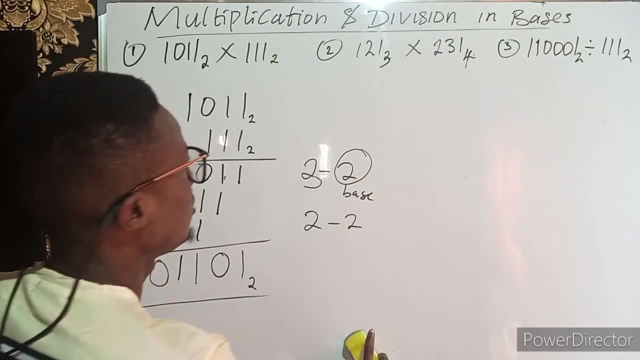 then i will write three plus. i'll write it over here. then i will write three minus third. this will give me a total of zero. so i'll write zero, base one, two. i've minus, i will call it one and transfer it over here. so this is just the answer to equation number one. okay, so let's go for. 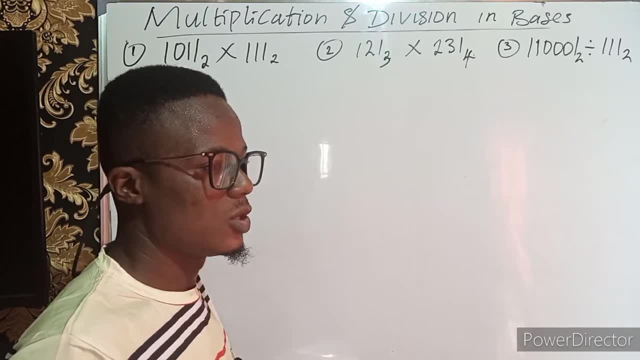 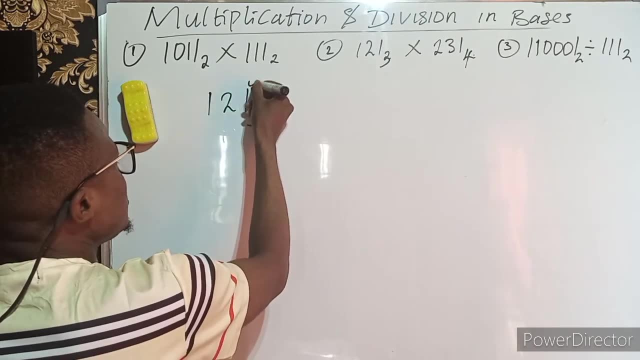 number two. in number two you can see that they are in different bases so you're not allowed to multiply them directly, so you've got to convert each of them to be stand for. the first number will have 3. here is 0, 25- base 3,��고com satisfactor: 2, base 3. 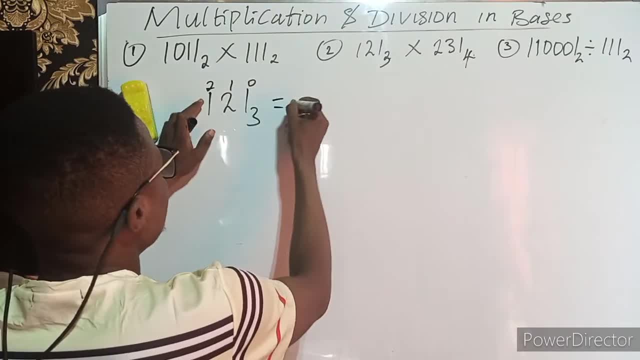 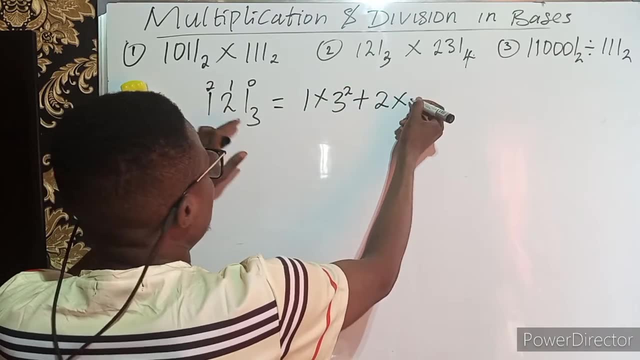 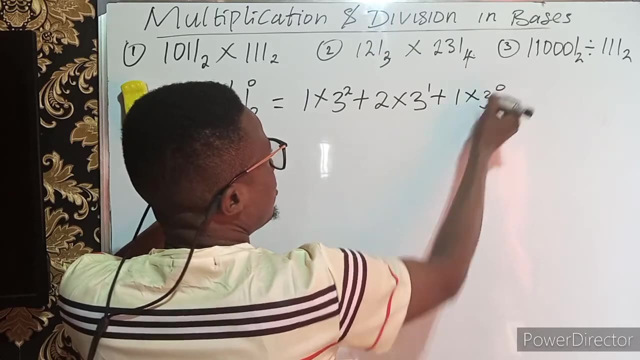 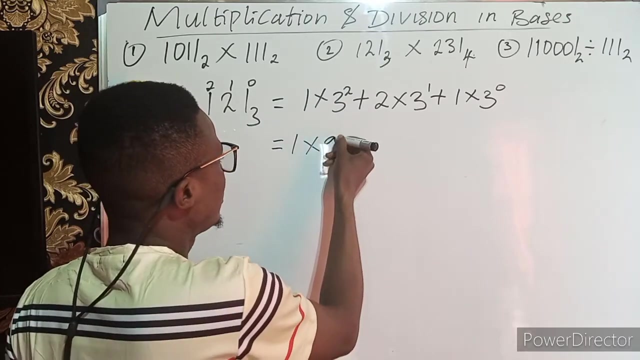 is 1, here is 2. so you say the first number is 1 multiplying by 3 power of 2 plus. the next number is 2 multiplying by 3 power of 1 plus. the last number is 1 multiplying by 3 power of 0. so this is something as 1 times 3 power of 2 is 9. 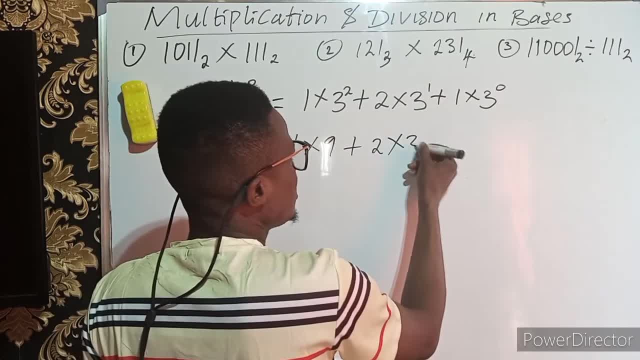 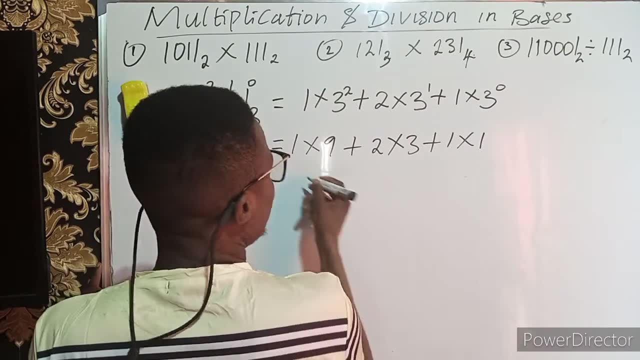 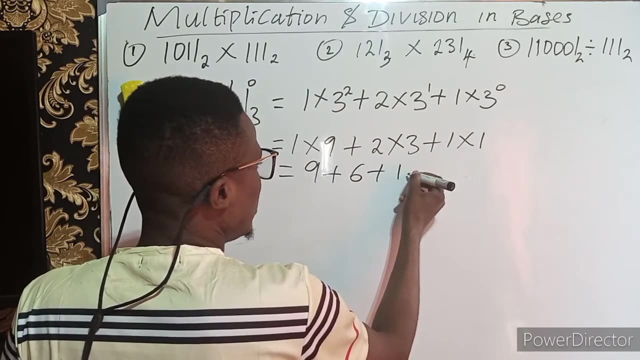 plus 2 times 3, power of 1 is 3 plus 1 times any number, power of 0 is a 1, so this simplifies to: 1 times 9 is 9 plus 2 times 3 is 6 plus 1 times 1 is 1. when 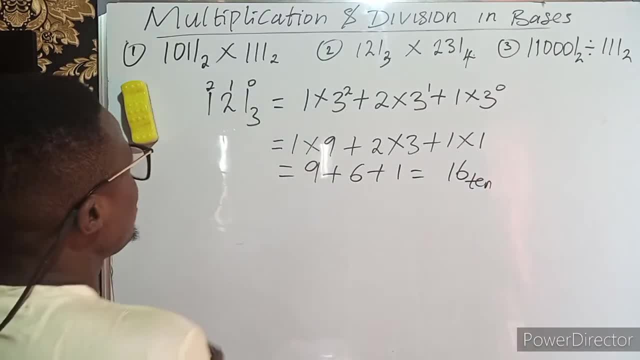 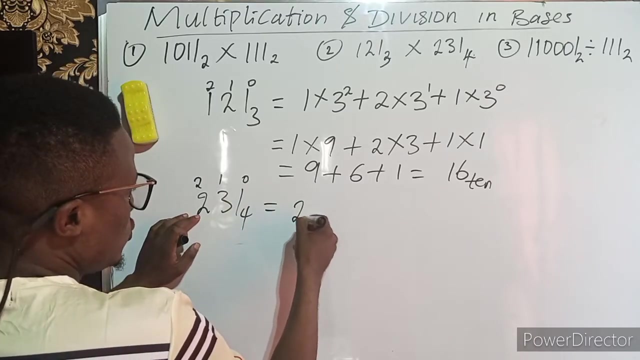 you add up, we get 16 in base 10. that's the equivalent of the equivalence of 1, 2, 1 base 3. so the next number is a, 2, 31, 2, 31, base 4. you still call here 0, 1 and 2, so this is now 2 times base 4, power of 2. 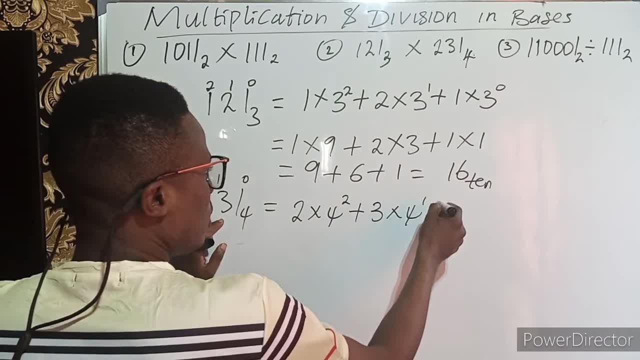 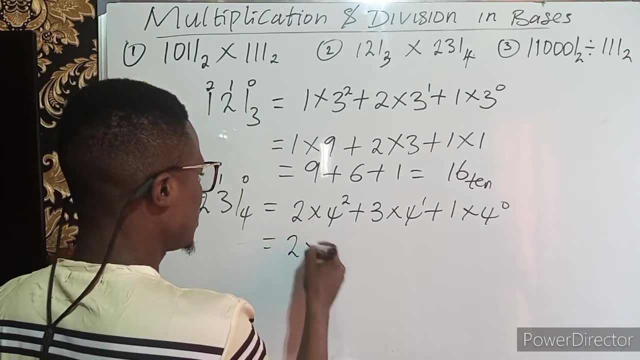 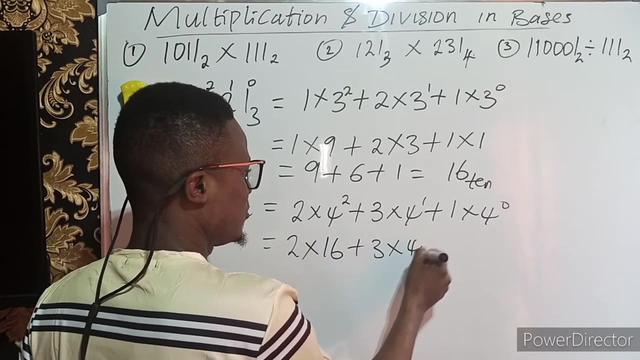 plus 3 times the base 4 power of 1, plus 1 times the base 4 power of a 0. so this is the something as 2 times 4 power of 2 is a 16, plus 3 times 4 power of 1 is 4. 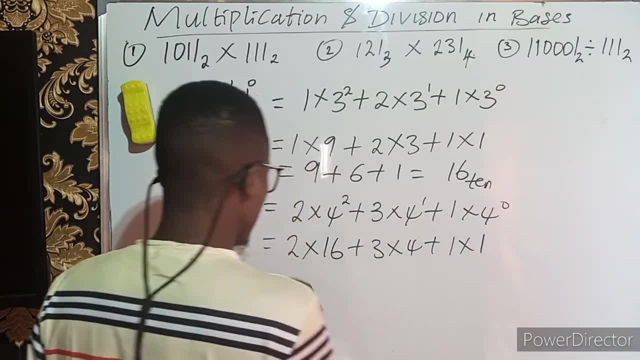 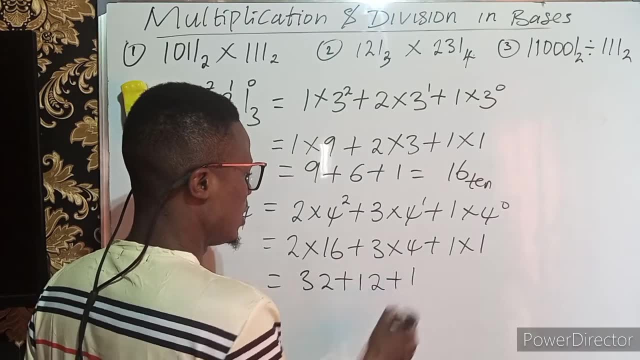 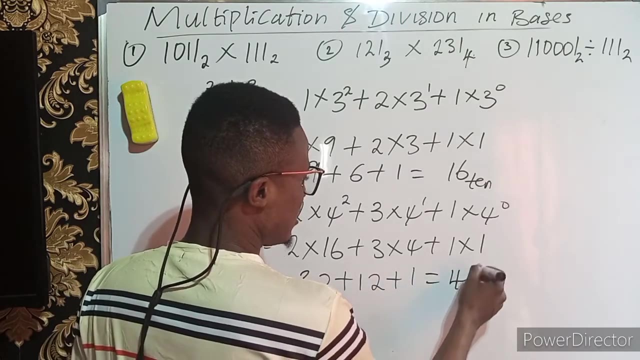 plus 1 times plus 1, any number power of 0 is a 1. 2 times 16 is 32, times 4 is 12, and 1 x 1 is 1. so 32 plus 12 is a 44 plus 1. we have 45 in base 10. then we are now free to multiply. 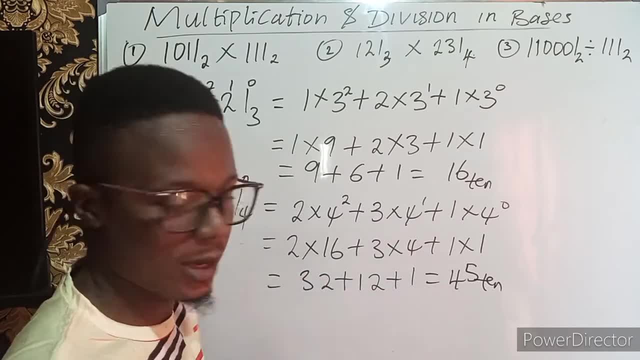 two of them. you can call it 16 in base 10, 4 times 5 plus 16 in base 10. that's the equivalent of 16 in base 10 x 45 in base 10, so 16 base 10 times 45 in base 10. so you correct me as. 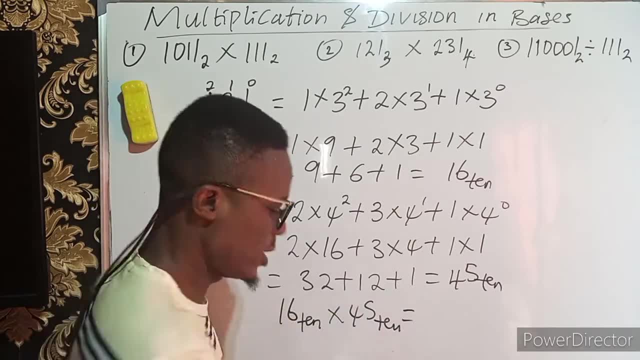 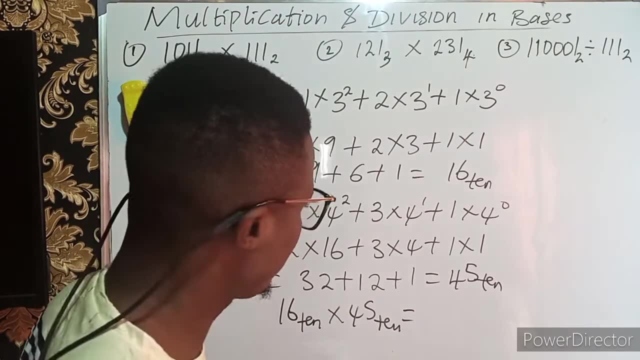 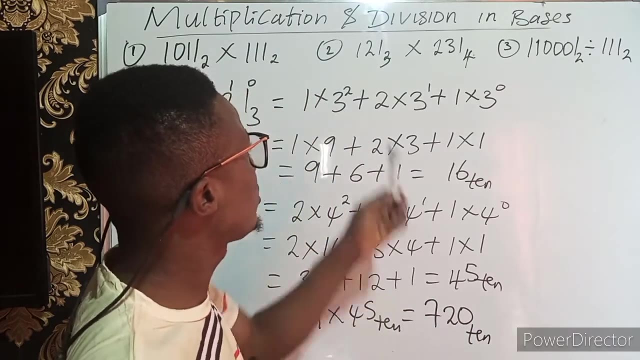 1, 4 or 3 times 4 negative, you get 1 and 3, 12. you are protected by 2 times 4 power of 1. let's use calculator and be fast: um 16 times 45 to give us 720, 720 base 10. now the examiner will. 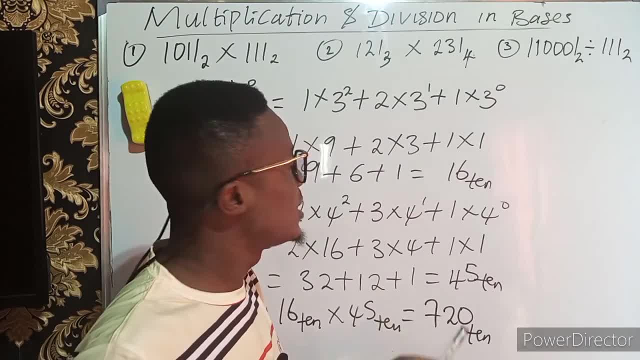 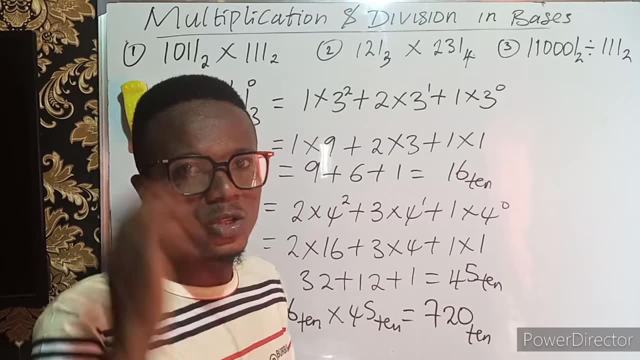 tell you the base you are going to leave your answer. so this is in base 10. the question can tell you to leave the answer either in base 3 or in base 4 or any other base they prefer. okay, so now, in this case, let us try to leave the answer in base 4, for instance, and see what it will give. 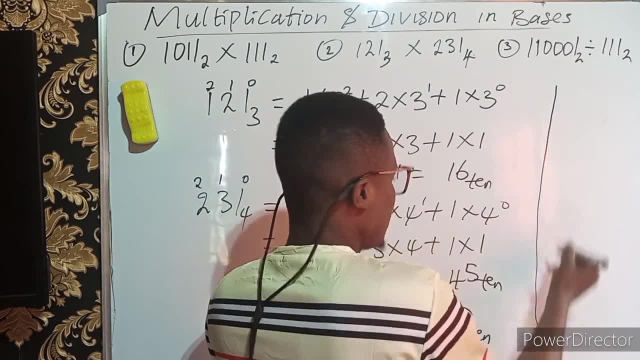 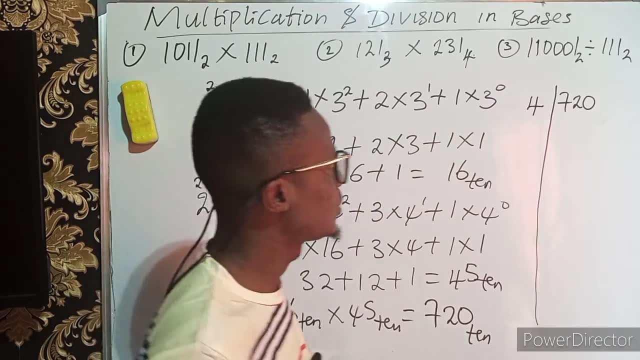 us to leave the answer in base 4. you've got to draw a straight line. you write 720, then you begin to divide by 4 because you want to keep the answer in base 4. okay, 4 divide 7 is 1, 1, remember 3. 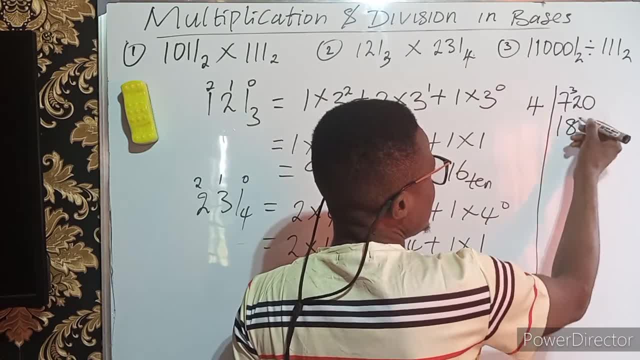 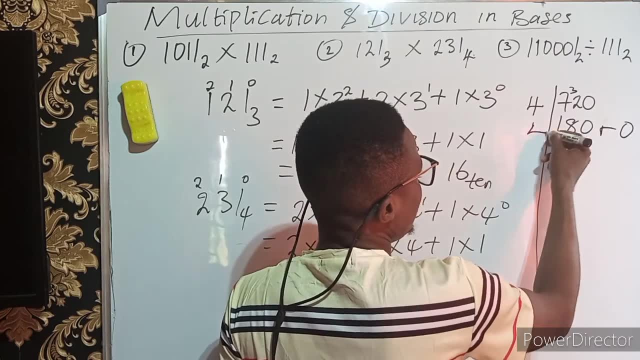 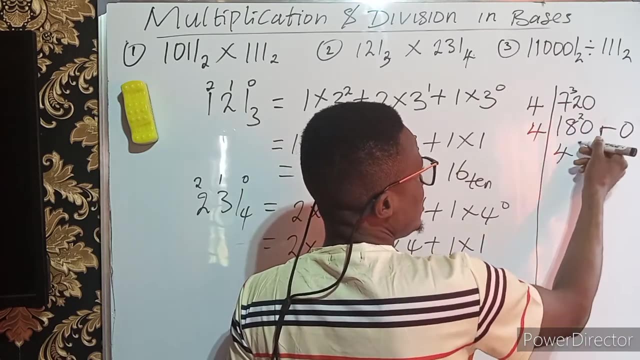 attach. it becomes 32. 4 divide 32 is 8 and 4 divide 0 is a 0 and there is no remainder. Use 4 again. 4 divide 18 is 4.. Remainder 2.. Our attachity becomes 20.. 4 divide. 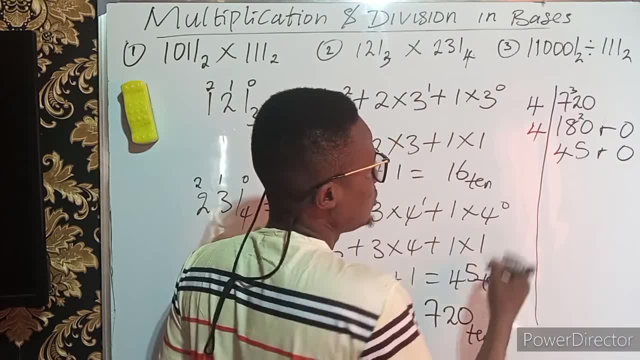 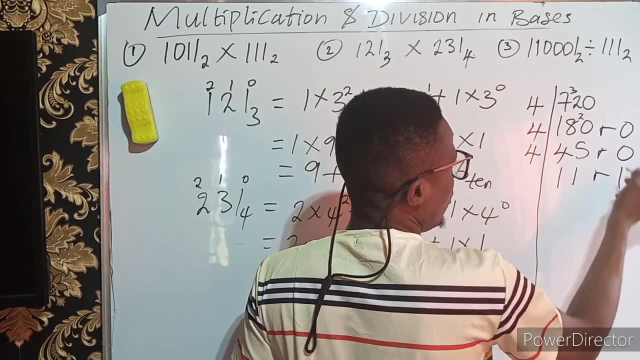 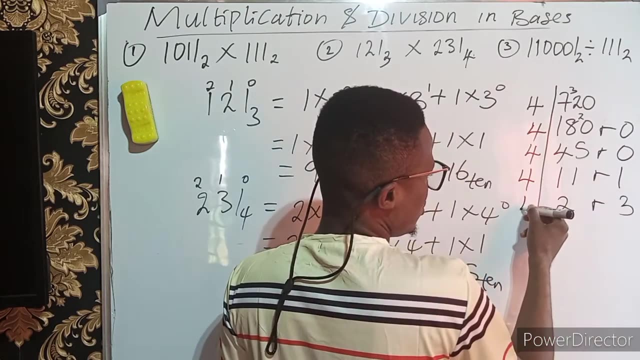 20 is 5.. Remainder 0.. I'll use 4 again. 4 divide 4 is 1.. 4 divide 5 is 1.. Remainder 1.. I'll use 4 again. 4 divide 11 is 2.. Remainder 3.. You continue using 4 because you are putting it in. 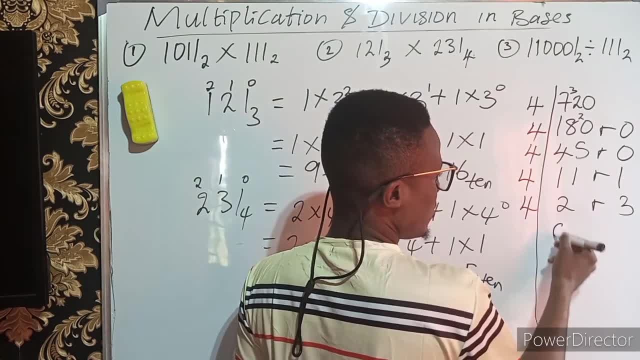 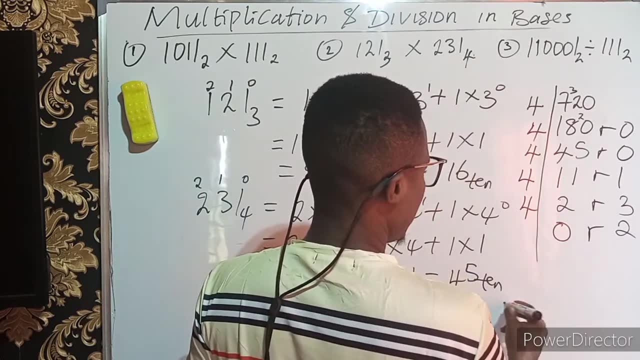 base 4.. If I divide 2 by 4,, 2 is now smaller than 4.. So I'll call it 0. Remainder whatever I'm having here, which is 2.. Then, if you now want to know your final answer, your final answer is: 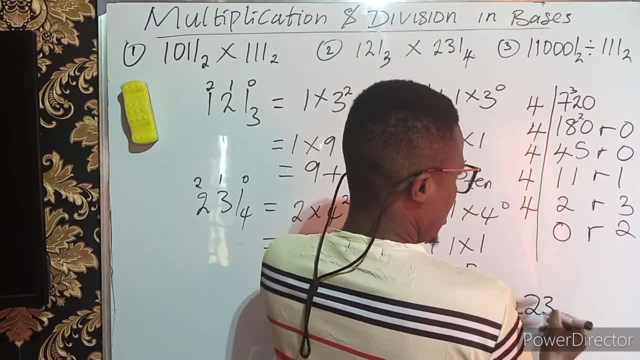 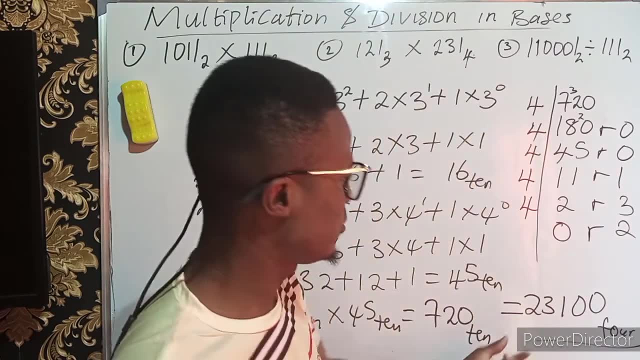 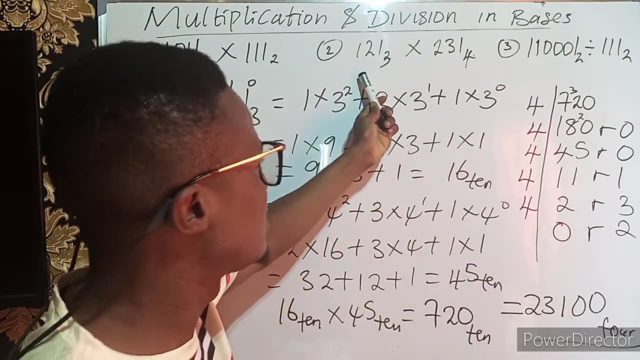 just starting from below here: 2 3 1 0 0- base 4.. 2 3 1 0 0- base 4 is now the answer. So I've just kept the answer to this particular question in base 4.. You can keep it in base 3 by dividing. 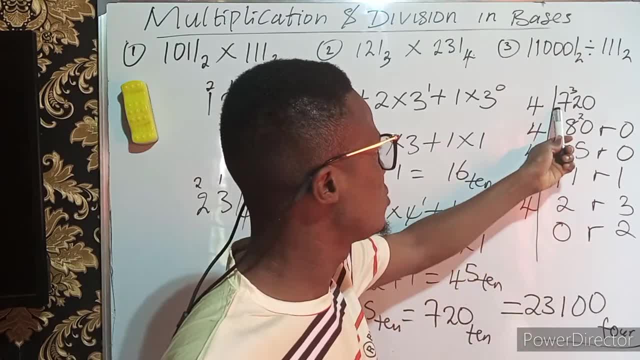 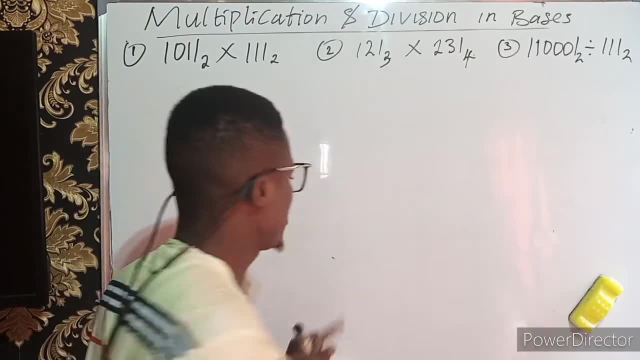 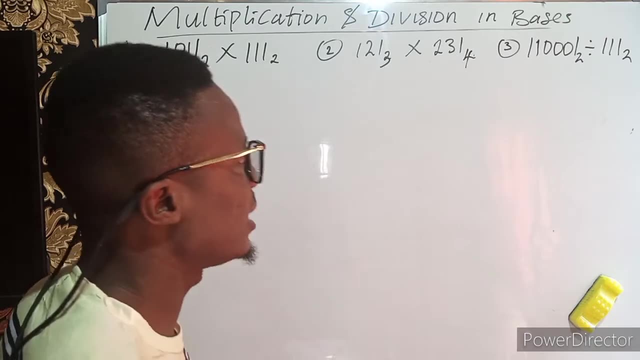 720 by 3.. You can keep it in any base you want by dividing 720 by that particular base. you want it to be Okay. so let's take the last question For division. you can divide directly, but that one is a big stress. So the best thing is to convert all of them to base 10 again, Then divide. 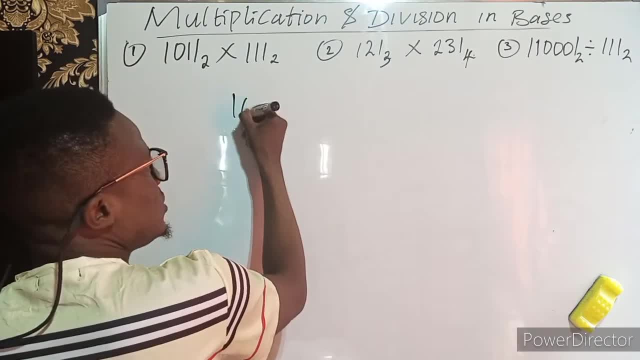 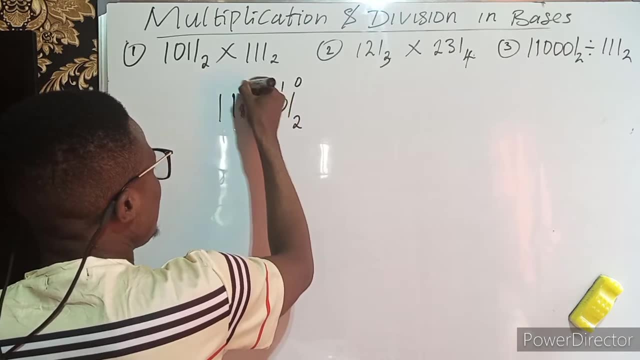 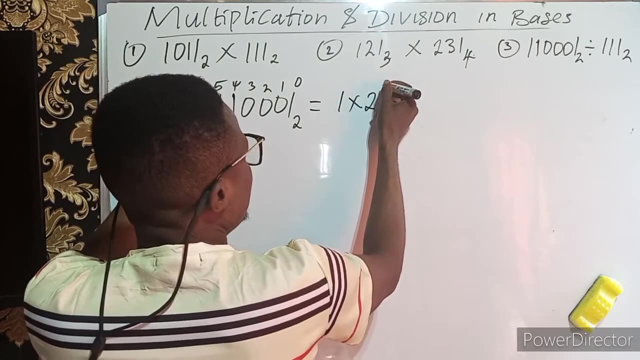 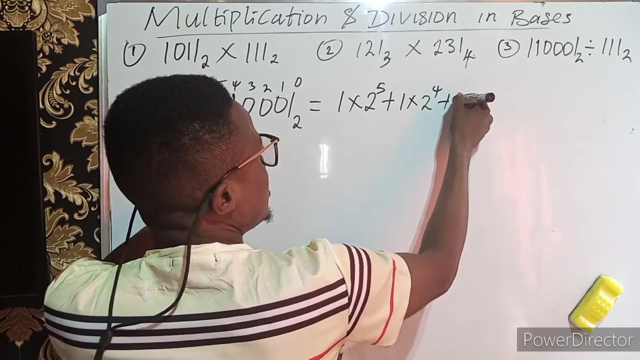 after bringing it back to base 2.. So we have 1: 0, 1, 1, 0, 0, 0, 1 base 2.. This is 0, 1, 2, 3, 4.. Under 5.. Okay, we'll call it 1 times base 2 power of 5 plus 1 times base 2 power of 4 plus 0 times. 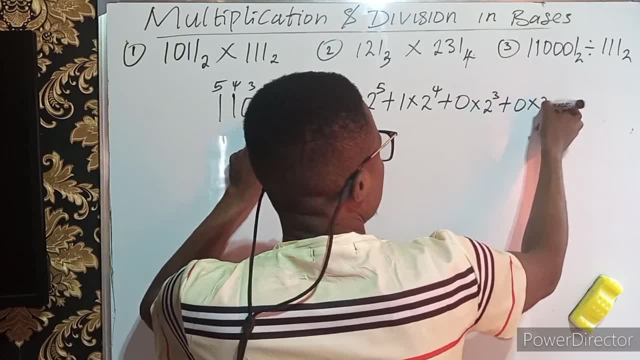 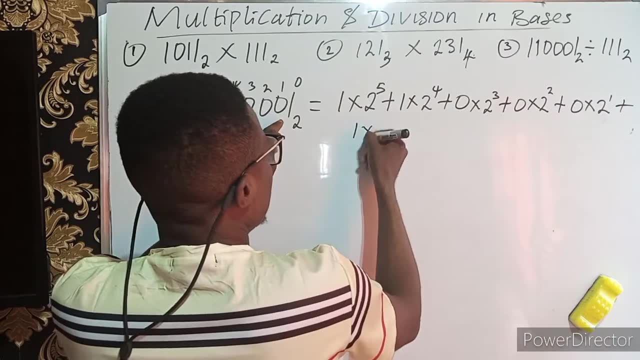 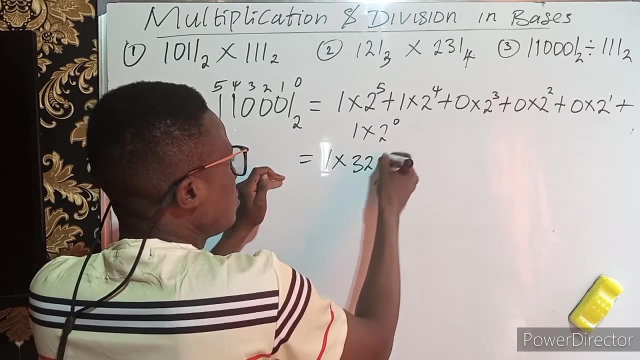 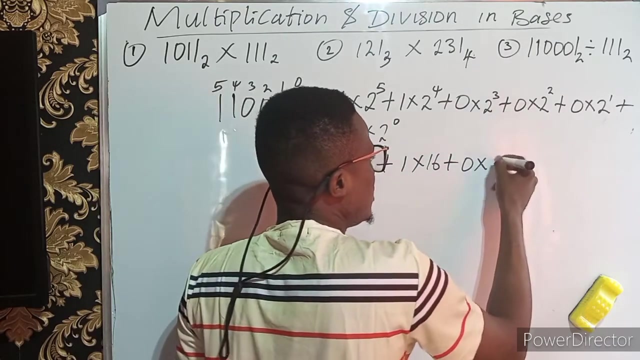 base 2 power of 3 plus 0 times base 2 power of 2 plus 0 times base 2. power of 1 plus 1 times base 2 power of 0. That gives us 1.. 2 power 5 is 32 plus 1 times 2. power 4 is 16 plus 0 times 2. power 3 is 8 plus 0. 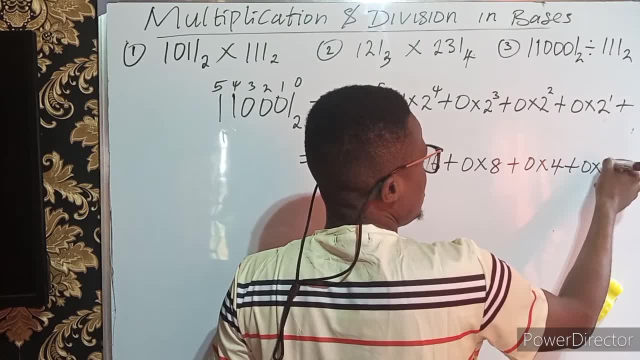 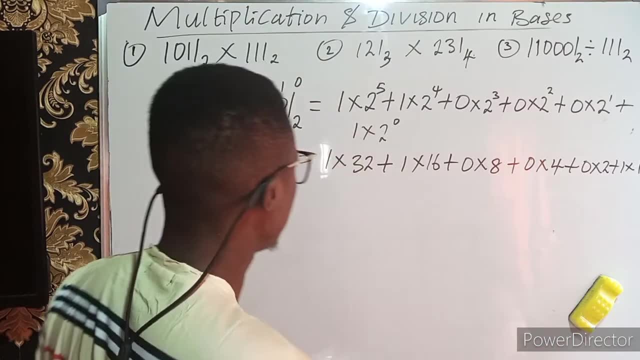 times 2, power 2 is 4 plus 0 times 2, power 1 is 2 plus 1. times 2, power 0 is 1, because any number power of 0 is 1. so this will give us: 1 times 32 is 32 plus. 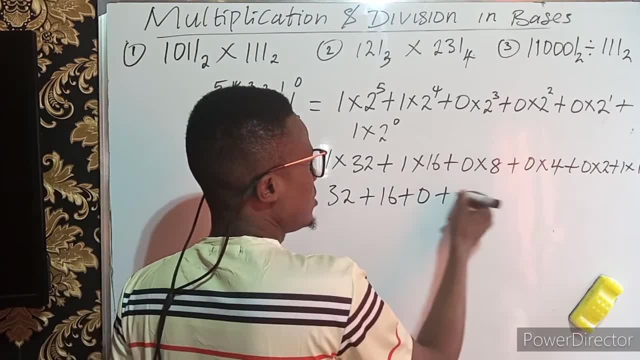 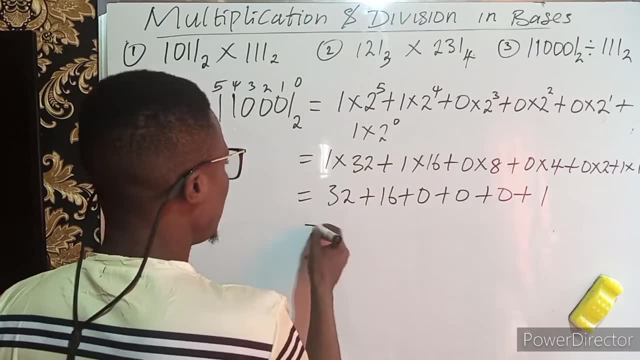 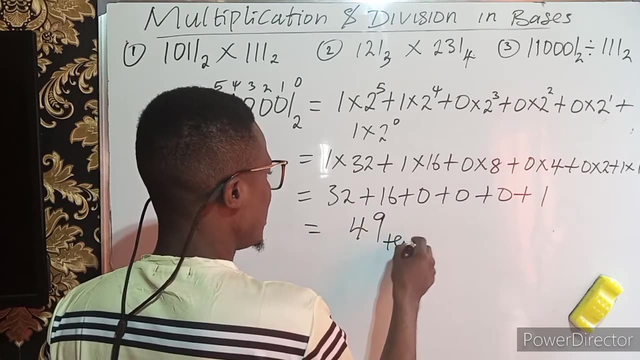 1 times 16 is 16, 0 times 8 is 0, 0 times 4 is 0. 0 times 2 is 0. 1 times 1 is 1. then you sum up: 32 plus 16 is 48. 48 plus 1 will give us 49. in base 10, we bring the: 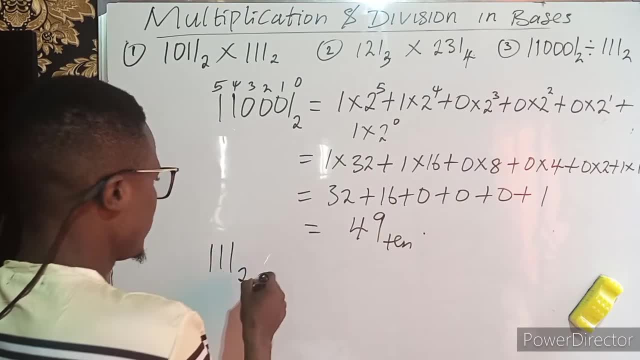 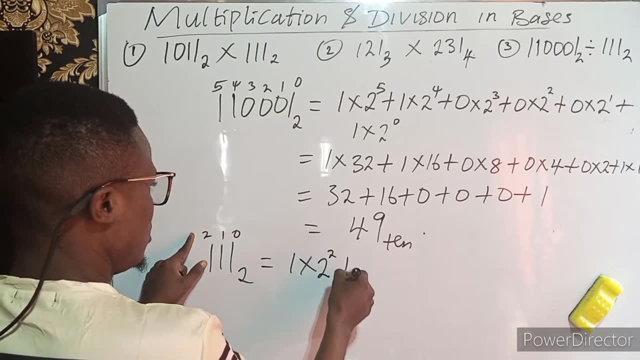 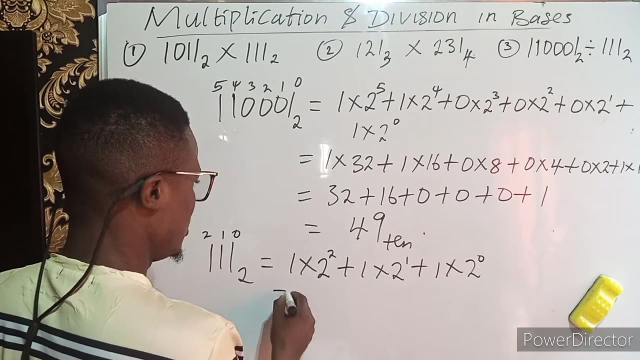 next number there, which is 1, 1, 1, 1, 1 1 base 2. you call here 0, 1 and 2, so you have 1 times base 2 power of 2 plus 1 times base 2 power of 1 plus 1 times base 2 power of 0. this is: 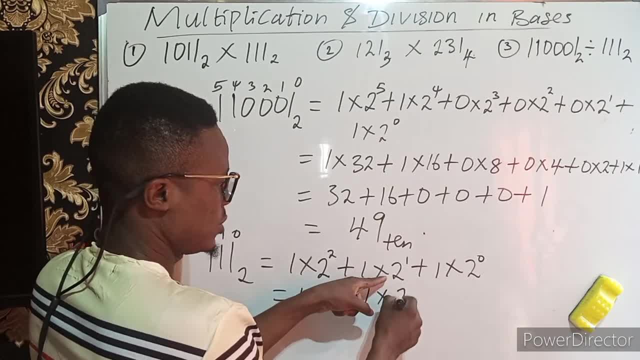 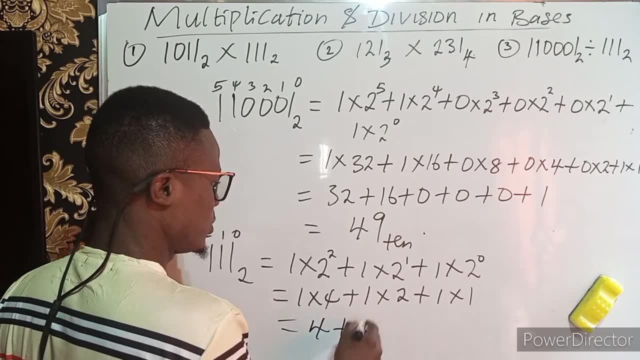 now, 1 times 4 plus 1 times 2 plus 1 times 1, any number power of 0 is 1. so 1 times 4 will give us 4, plus 1 times 2 will give us 2. 1 times 1 will give us 1. 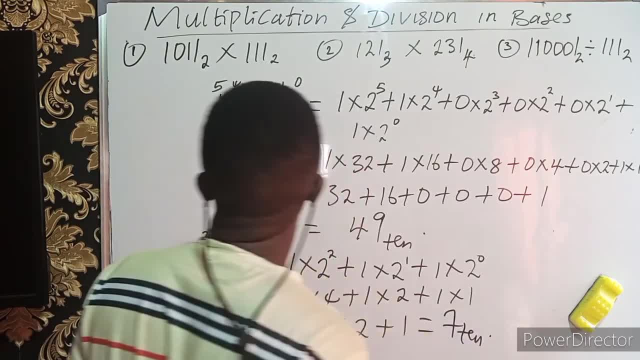 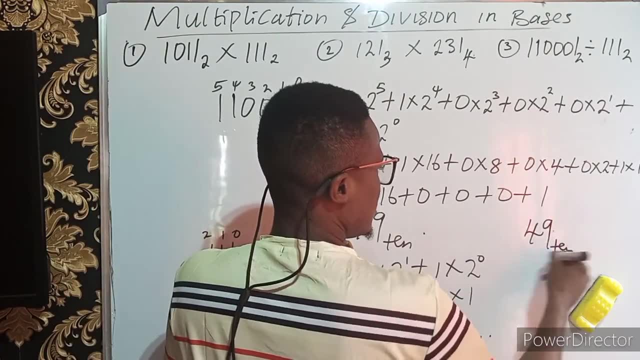 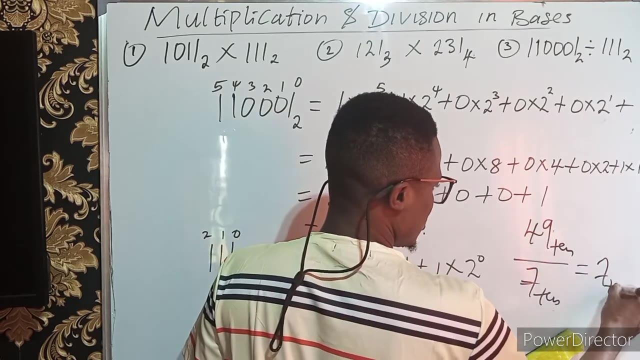 when we add up, this will give us 7 base 10, but we are asked to divide, so we've just got to say the first one, which is 49 base 10 divided by 7 base 10. and of course, when I divide 49 by 7 is giving me 7, also 7 base 10. so but the answer? 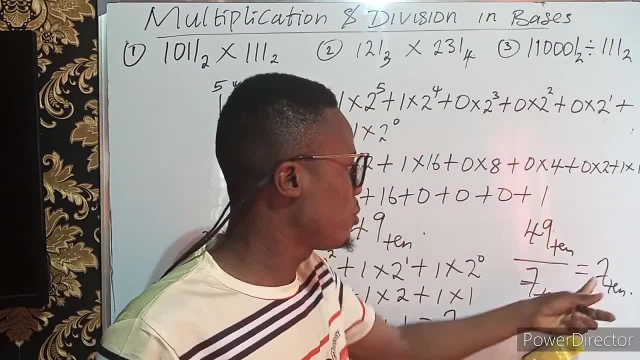 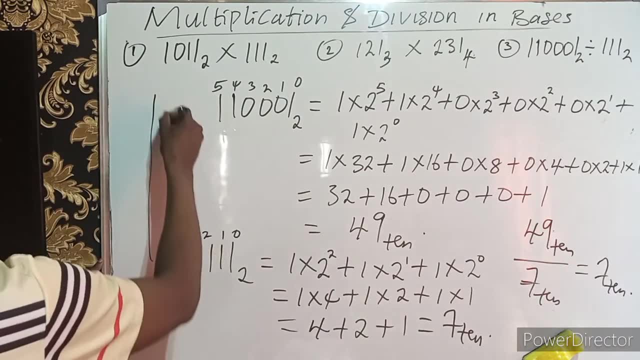 shouldn't be in base 10, since they have uniform basis base 2. so we are going to convert 7 in base 10 to base 2 and that will be our final answer. so you just draw a straight line and write 7, you start dividing by 2 and taking the 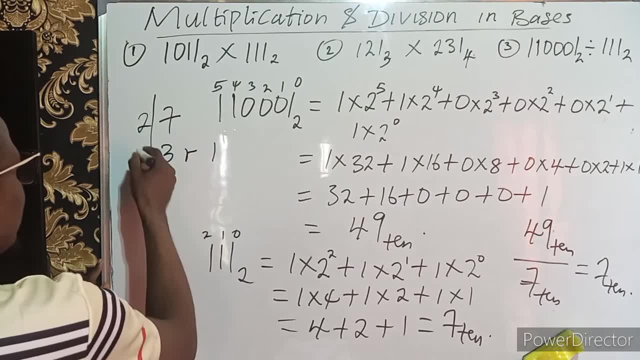 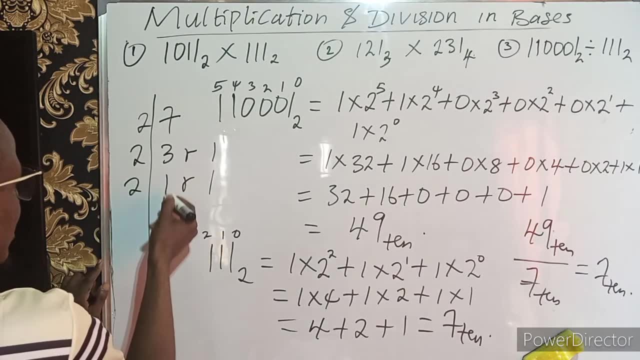 remainder. 2 divided by 7 is 3 remainder 1. 2 divided by 3 is 1 remainder 1 and 2 divided by 0, 2 is now bigger than 0. you call it 0 remainder 1. so you count from down to up. 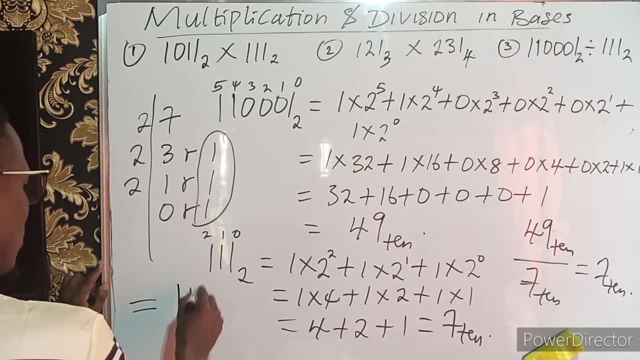 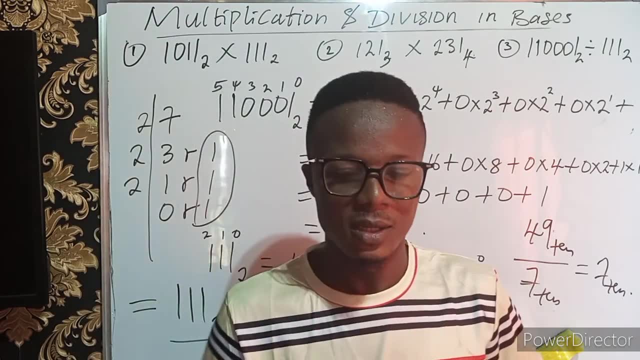 answer is now: 1 1 1 1 1 1 base 2. this is just the answer to this question. so you've seen how to multiply and divide in basis. thank you. 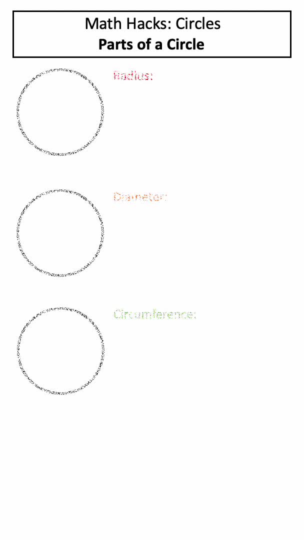 Hi, there. today we're covering the different parts of a circle and the formulas we use to calculate them. The radius is the distance of a line segment from the center of the circle to the circumference, and it can be calculated using the formula shown here. 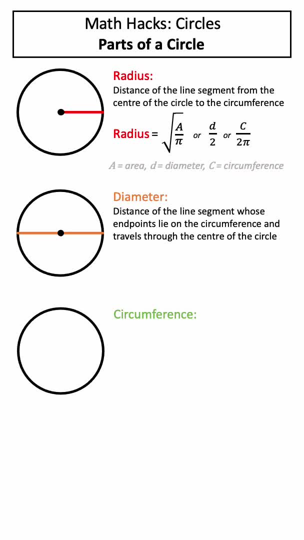 The diameter is the distance of the line segment whose endpoints lie on the circumference and travels through the center of the circle, and it can be calculated using the formula shown here. The circumference is the distance around a circle, and it can be calculated using the formula shown here. 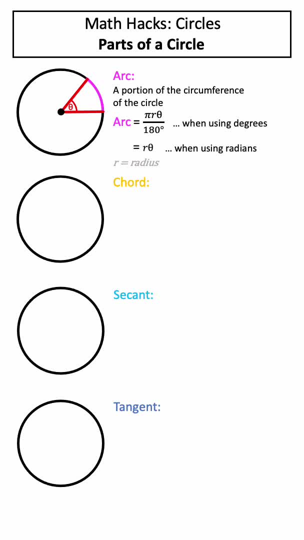 An arc is a portion of the circumference of the circle and can be calculated using the formula shown here. A chord is a line segment that joins two distinct points on a circle circumference, and it can be calculated using the formula shown here. A secant is a line that intersects the circle at two different points and a tangent is.